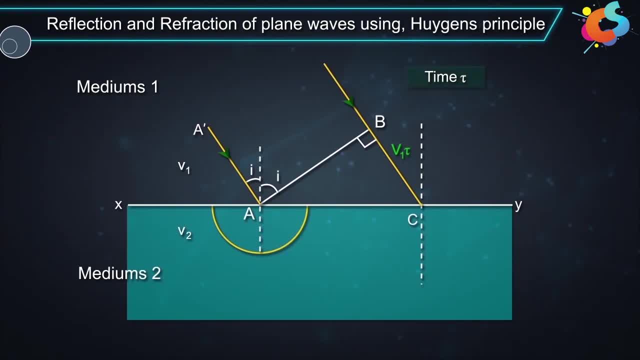 sphere of radius v2 tau from point A in medium 2.. Now draw a tangent plane from point C to the sphere. We will call this point as E. This plane, CE, represents the refracted wave front and the angle ACE is equal to R, represents angle of refraction. 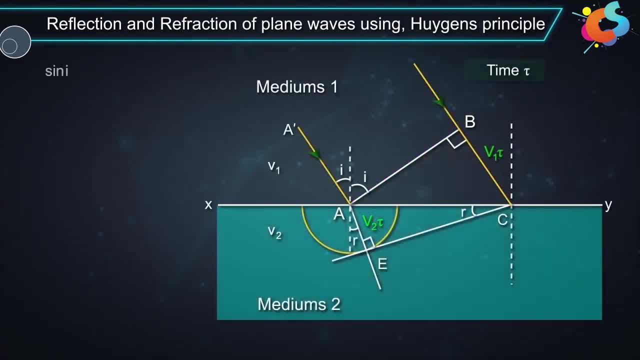 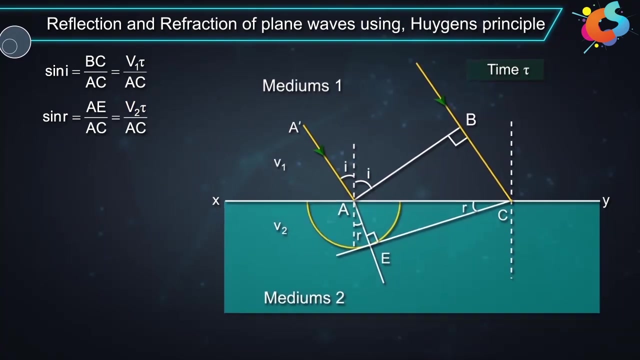 From triangle ABC, sine I is equal to BC by AC, which is equal to v1 tau divided by AC, And from triangle AEC, sine R is equal to AE divided by AC, which is equal to v2 tau divided by AC. Therefore, sine I divided by sine R is equal to V2 tau divided by AC. Therefore, 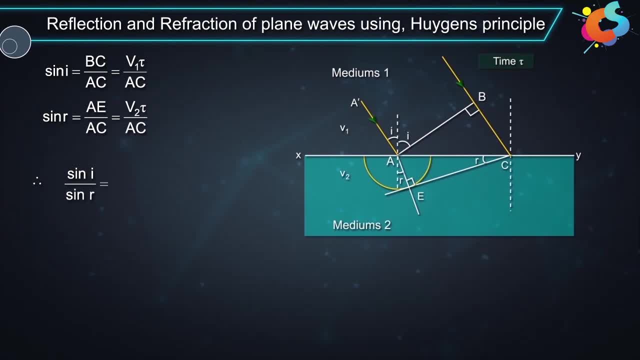 Therefore, sin I divided by sin R is equal to V1 tau divided by AC. whole divided by V2 tau divided by AC, This is equal to V1 by V2.. Since V1 is constant in medium 1 and V2 is constant in medium 2, we have sin I by sin R is equal to V1 by V2, which is equal to. 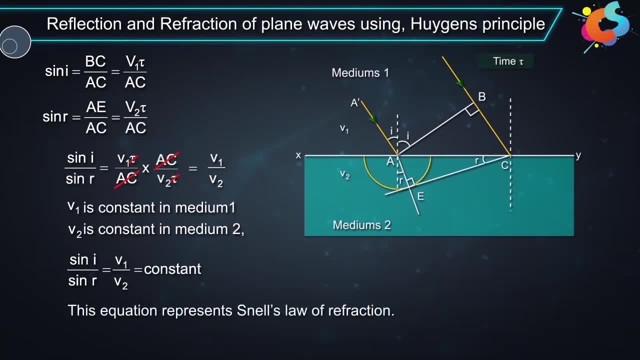 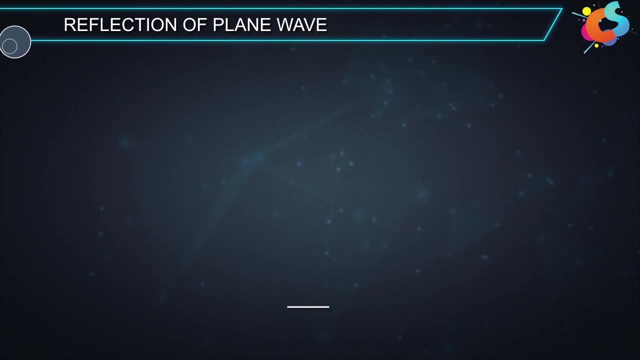 a constant. This equation represents Snell's law of refraction. Reflection of a plane view. Consider a reflection surface XY. Now let a plane wavefront, AB, be incident on the reflecting surface at an angle I. The secondary wavelet from B will strike the surface XY at point C in time, tau. Then 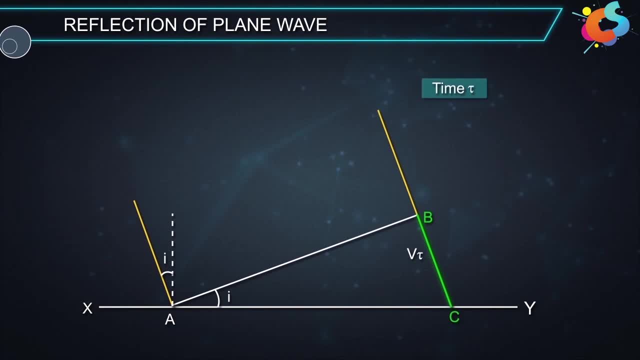 BC is equal to V tau. At the same time, the secondary wavelet from A will get reflected and travel the same way. At the same time, the secondheus of B will return at the same distance. V tau in the same medium, 13 met, absorbing V4�� to the centre of the reflective surface, which is